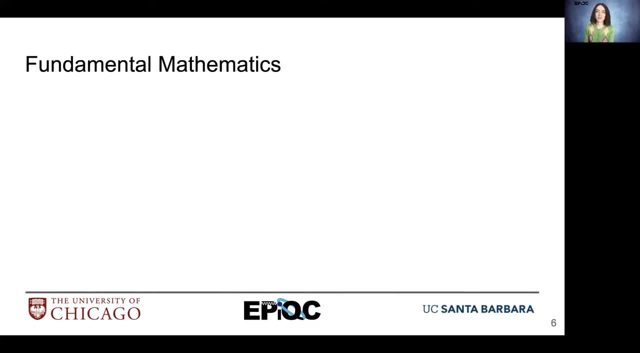 that large number, n. Let's talk about some fundamental mathematics that we'll need to understand. Shor's algorithm To decrypt data. first we need to know the prime factors of our target number, n. So for n equal to g times h, we want to determine some g, The guess. 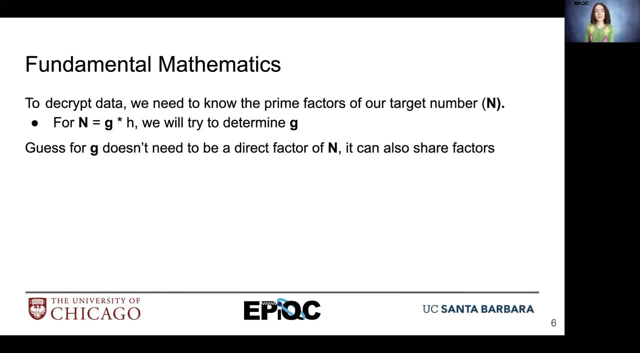 that we have for g doesn't need to be a direct factor of n. It can also share factors. That's because we can have the case where n is equal to a times b and g is equal to a times c. So therefore we have a accessible to us which is a factor of n, For example. we can 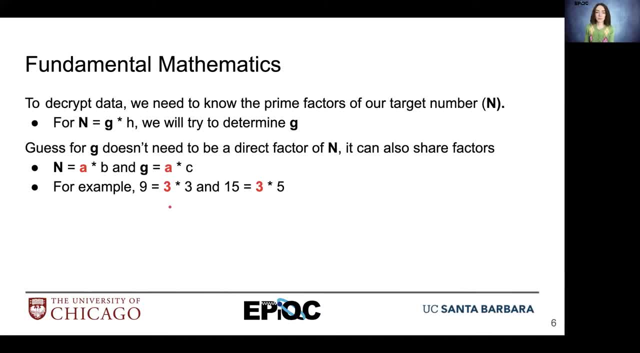 have 9 equal to 3 times 3 and 15 equal to 3 times 5.. They both share a factor of 3,, even though 9 is not a direct factor of 15.. The largest value that divides two numbers with no remainder is called the greatest common factor. 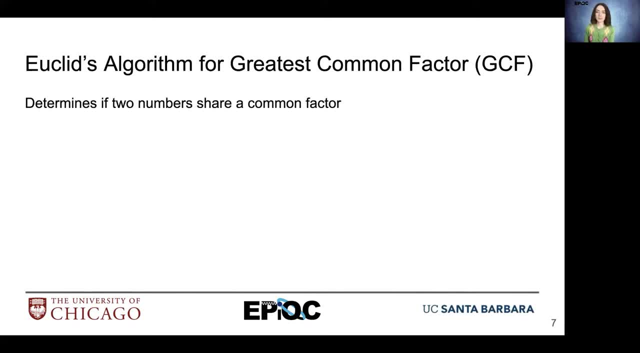 We'll call that the greatest common factor. We'll call that the greatest common factor. We'll call that the greatest common factor. We'll call this the GCF. Euclid's algorithm can help us to determine a greatest common factor for two values. When we use it, it helps us determine if these two values share. 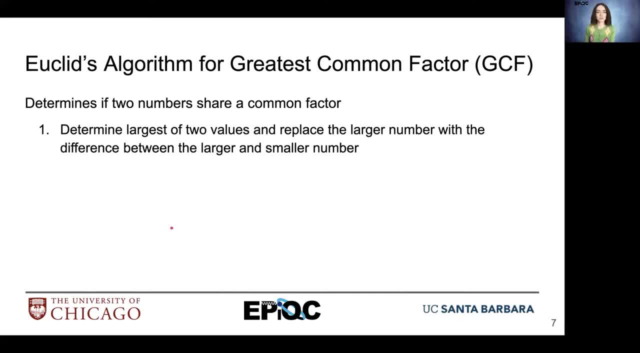 a factor. The procedure is as follows: We determine the largest of two input values and replace the larger number with the difference between the larger and the smaller. We repeat until one of the values becomes zero or the two arguments are equal. At that point, the 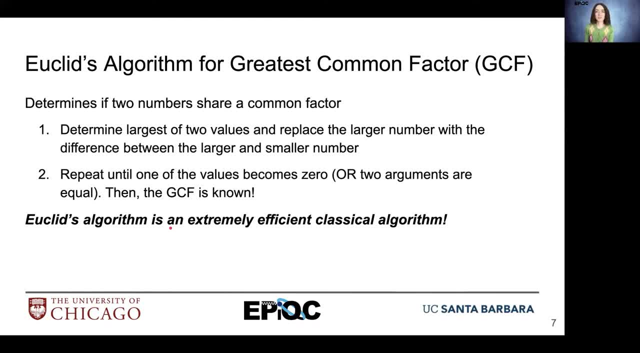 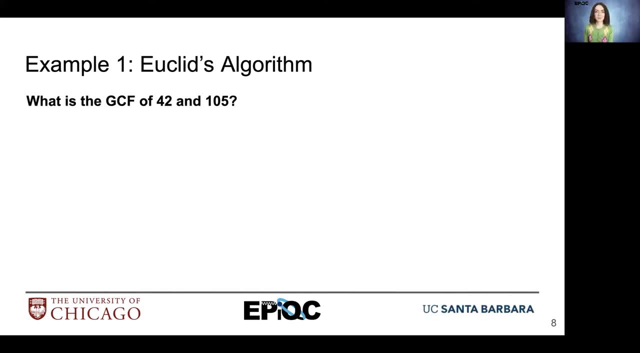 Euclid's algorithm is incredibly useful and it's extremely efficient to implement classically. Let's do an example. What is the greatest common factor of 42 and 105?? Well, we first determine the larger of the two- so that would be 105, and subtract the smaller from the larger. 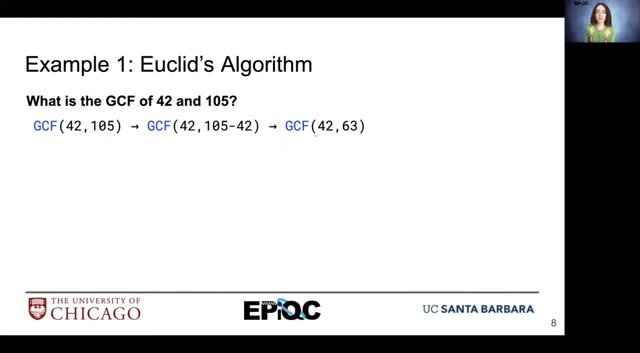 That transforms 42 and 105 to 42 and 63. We repeat the procedure. First we determine the greatest common factor, so that would be 53, and subtract the smaller from the larger until our numbers get smaller and smaller. At this point, when we have 0 and 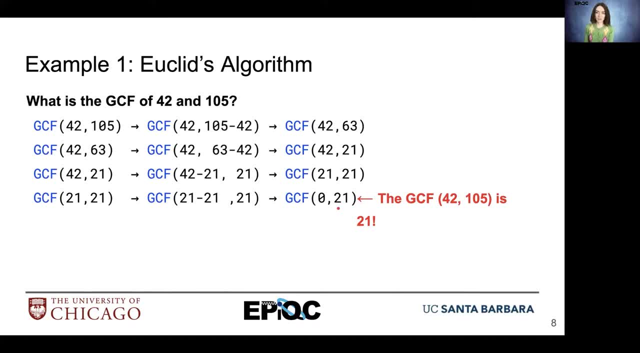 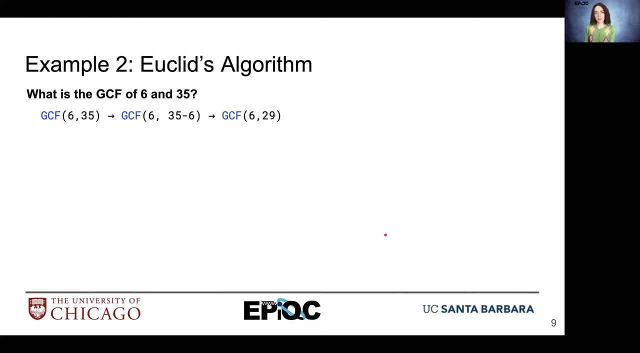 21,. we stop. We know that our greatest common factor of 42 and 105 is 21.. Let's do another example: What is the greatest common factor of six and 35?? First, we determine the largest number out of six and 35, and we subtract some of that. We also determine: 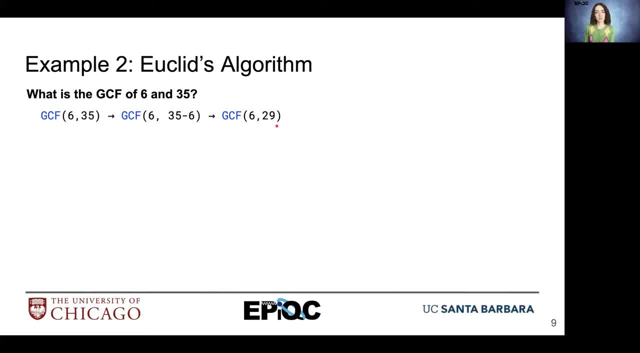 tract smaller. So 35 minus 6 gives us 29.. 29 minus 6 gives us 23.. 23 minus 6 gives us 17.. 17 minus 6 gives us 11.. We continue this routine until we reach two equal values. The greatest common factor of 6 and 35 is 1.. 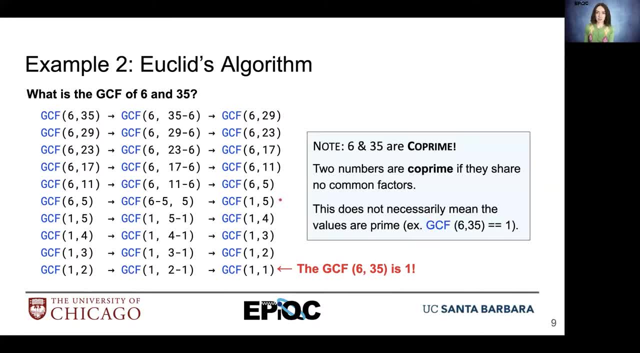 What does that mean? Since 6 and 35 share no other factor besides 1,, that means that the two values are co-prime. This doesn't necessarily mean that the values are prime themselves. For example, a factor of 6 is 3 and a factor of 35 is 5.. Guessing a direct. 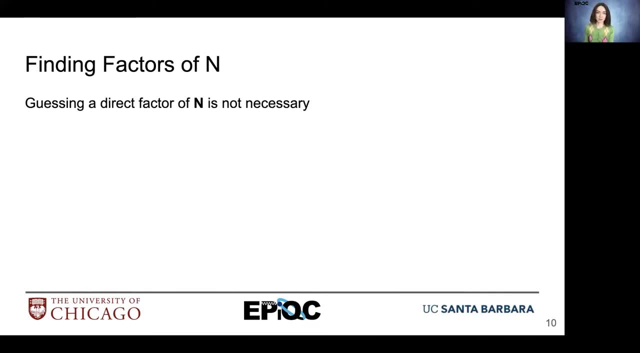 factor of n is not necessary when we're trying to factor n itself. We just saw with Euclid's algorithm that we just have to find something that shares a factor with n and we're good to go. It will still enable us to decrypt our secret messages. What we can do is we can apply. 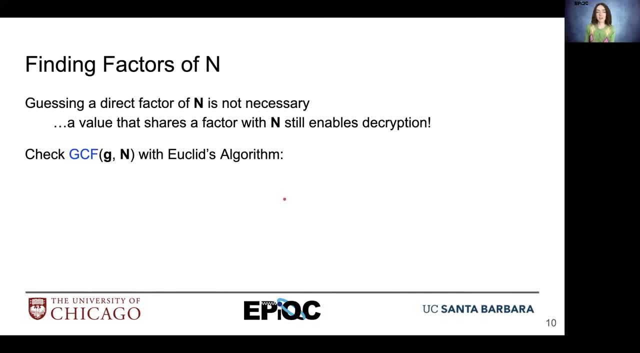 Euclid's algorithm and check if our guess g shares a factor with n, If the greatest common factor of g and n is not equal to 1, in other words they're not co-prime. we found a factor of n and we are done. We can use g and n divided by g to decrypt our message, because n divided by g will. 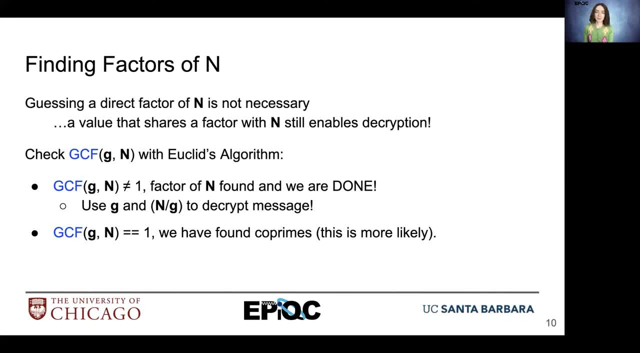 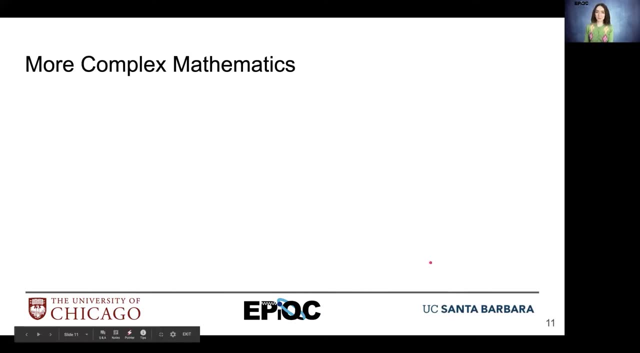 give us our factor of n. If our greatest common factor of g and n is equal to 1, we have found co-prime values. This is more likely. unfortunately, If we find co-primes, we need to do more processing. in order to improve our guess for g, Let's introduce some more complex mathematics. that'll. 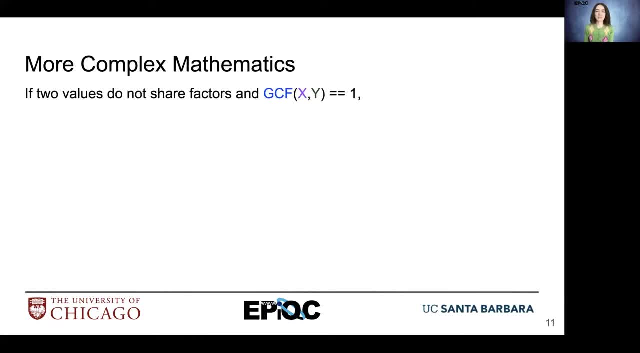 help us find a better guess for g If two values do not share factors. so in this example we'll look at x and y. they'll be co-primes and their greatest common factor is equal to 1.. So we can take our co-primes x and y and relate them in such a way that we can take x multiply. 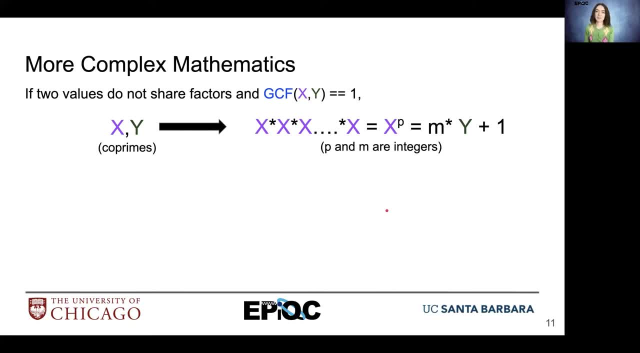 it by itself many times, or in other words, raise it to some exponent p and that'll be equivalent to m, some constant times y plus 1. Here p and m are both integers. Let's try this So for our example, that we previously 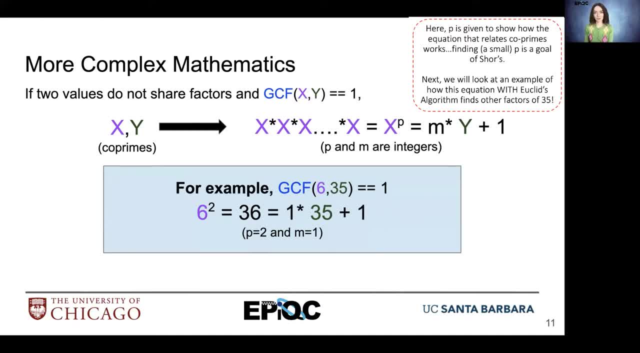 worked where the greatest common factor of 6 and 35 were equal to 1,. we can take 6,, raise it to the 2, and that's equal to 36.. It's also equal to 1 times 35 plus 1.. So, using this relation, we just 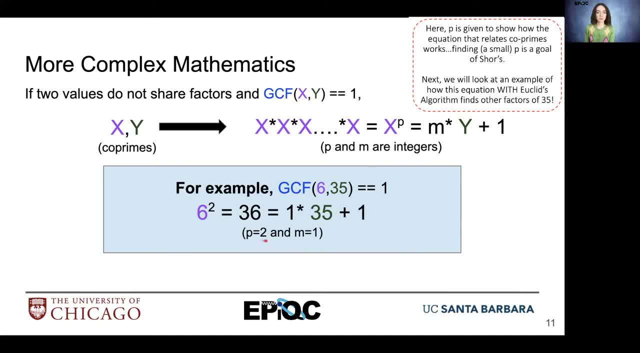 described, we found that p can be equal to 2 and m can be equal to 1 in order to relate the co-prime values of x and y. This technique works for any set of co-primes. Using that earlier logic, we just 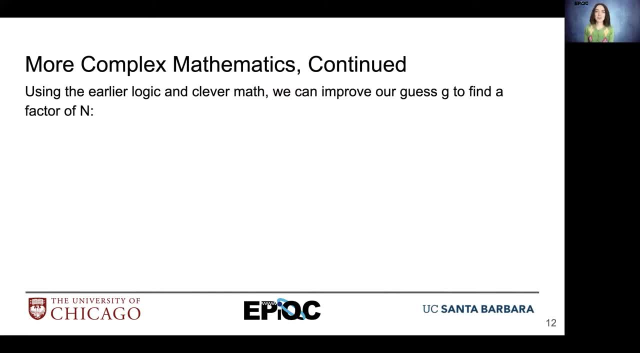 described, we can improve our guess for g and n If we find co-primes of x and y. we need to change our guess of g in order to find a factor of n. So here we have g raised to, the p is equal to. 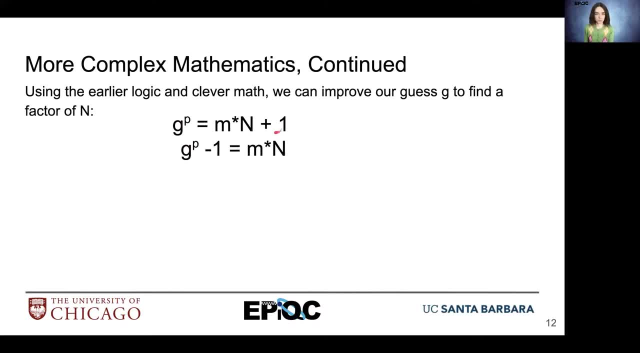 m times n plus 1.. Let's move that one over to the other side of the equal sign and we're able to expand the left side of our equation in order to find g raised to the p over 2 plus 1, times g to the p over 2 minus 1, is equal to m times n. We can check with foiling to see that g. 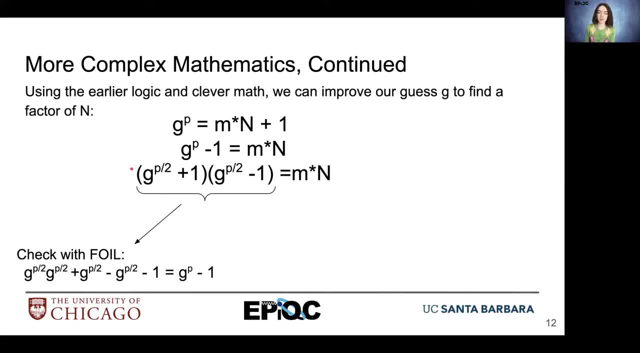 both of these expressions are equivalent that are on the left of the equal sign. These terms produce improved guesses for factors of n because of Euclid's algorithm. Remember, we don't necessarily need to find a direct factor of n, we just need to find something that shares. 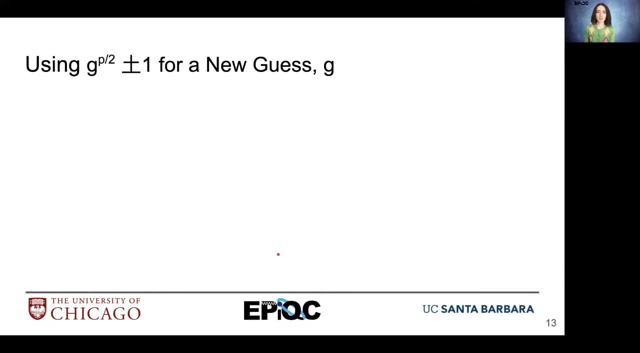 a factor. So let's improve our guess for g using the term we just defined: g raised to the p over 2 plus or minus 1.. In our previous example, when we looked at n equal to 35 and g equal to 6,, 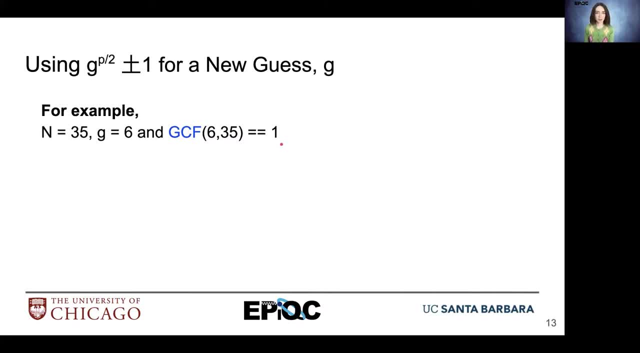 we saw that they did not share any factors. They were co-prime because the greatest common factor with Euclid's algorithm was equal to 1.. For p equal to 6, we have 6 raised to the 6 divided by 2. 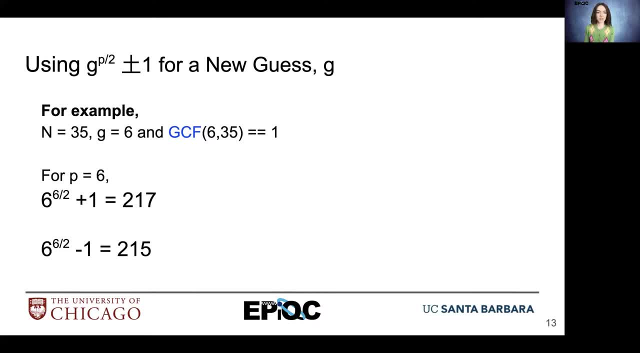 plus 1, equal to 217.. And then we have 6, raised to the 6, divided by 2 minus 1, equal to 2.. And then we have 6, raised to the 6, divided by 2 minus 1, equal to 1.. 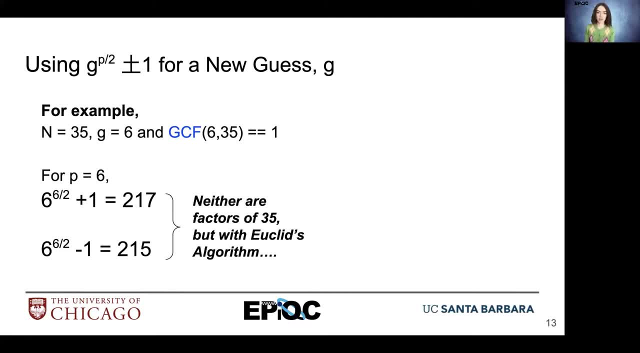 Neither of these are factors of 35, but luckily we have Euclid's algorithm. The greatest common factor of 217 and 35 is 7, and the greatest common factor of 215 and 35 is 5.. With these factors, 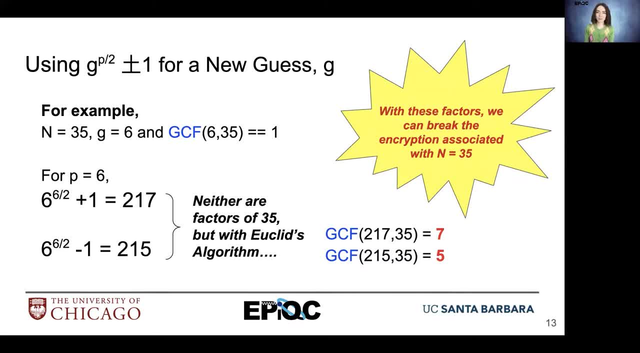 we can break the encryption associated with n equal to 35.. Although this is a trivial example and in reality our encryption would use much larger integers. this just goes to show the effectiveness of the Euclid's algorithm. We can break the encryption associated with n equal to. 6, so we have 6 raised to the 6, divided by 2 plus 1, equal to 217, and the greatest common factor of 217 is 7, and the greatest common factor of 217 is 5.. This is a very important 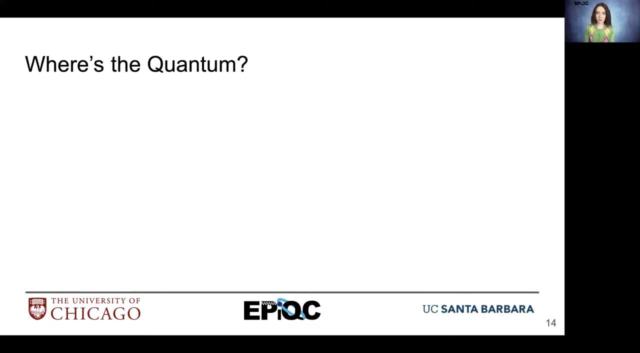 factor in Euclid's algorithm. So this is all about the effectiveness of these techniques that are included in Shor's algorithm. So one may ask: where's the quantum in all of this? There's still the challenge of finding the right exponent p for g raised to the p divided by 2. 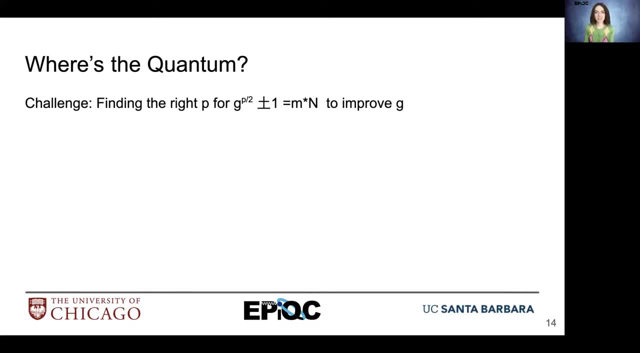 plus or minus 1, that is equal to some constant m times our integer of interest, n, And we need that value of p to improve our guess g. Not every p will work. We have a couple of constraints we need. we need to consider: For example, we don't want a p-value that will produce a multiple of n, We only 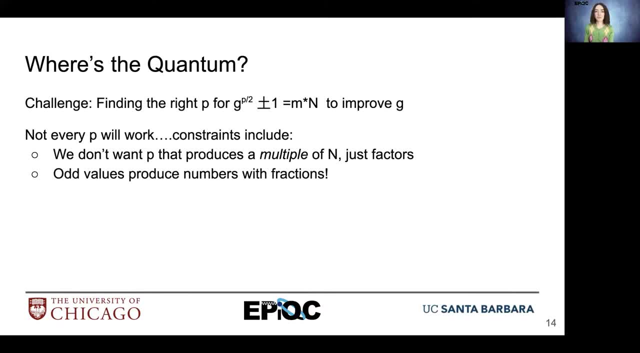 want factors. Additionally, odd values produce numbers with fractions, so we want to avoid those as well. As n gets larger, our search space for p increases dramatically, so testing many values of p would take a long time classically. Think once again about that guess-and-check technique. we'd 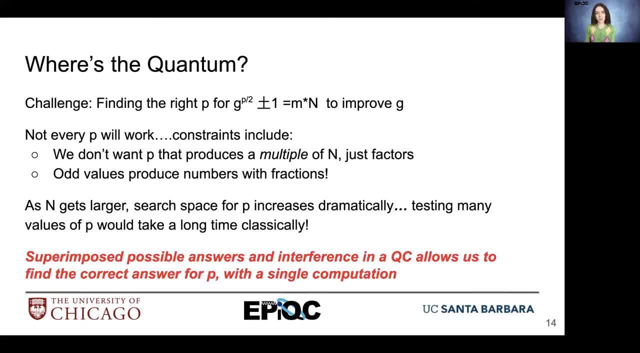 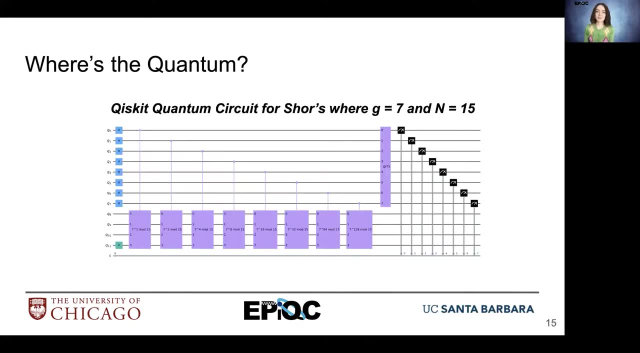 have to implement. Lucky for us, quantum computers implement superposition and have interference between signals, so superimposed possible answers combined with interference will allow us to find the correct answer for p within a single computation. Here we have an example implementation using Qiskit for the quantum circuit part of Shor's algorithm, where g is equal to 7 and n.